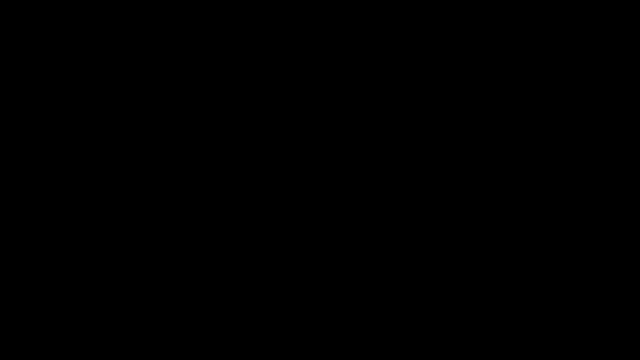 In this video, we're going to talk about exponential growth and decay problems as it relates to population growth, so to speak. Now, the first equation you need to be familiar with is this equation: dp divided by dt is equal to k times p. 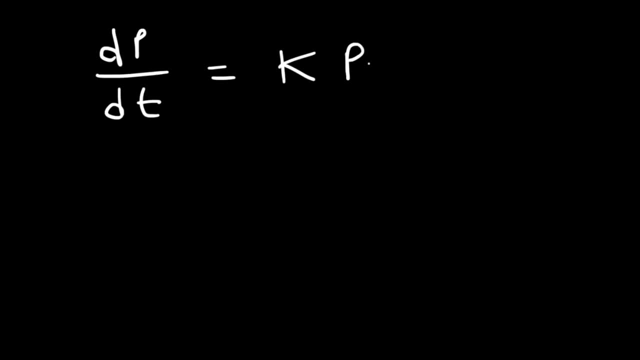 So this equation tells us that the population grows at a rate that is proportional to the size of the population. The population growth rate is dp by dt. That's how fast the population is growing at a given time. k is the relative growth rate and p is the size of the population at some time t. 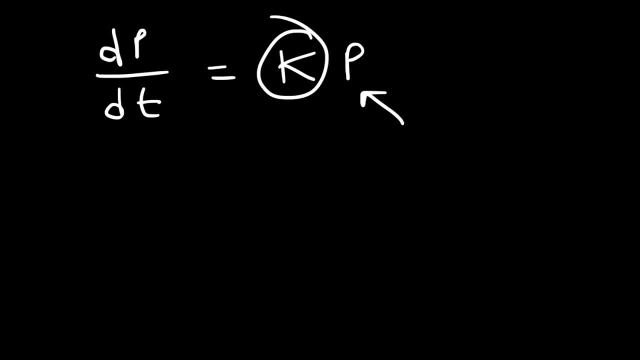 Now to understand this conceptually. let's say if we have a sample of a thousand bacteria, Okay, Okay. And let's say that in this sample the bacteria grows 50 cells per hour. What's going to happen if we double the population? 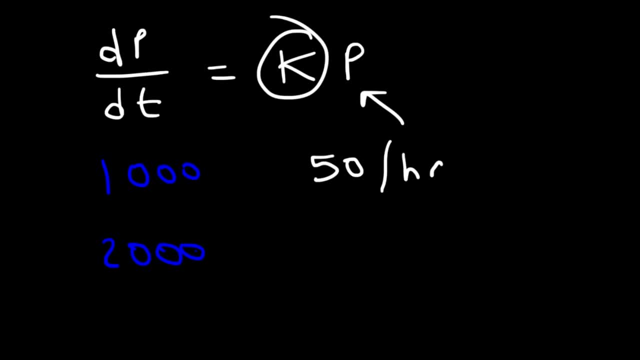 Let's say, if we have a sample of 2,000 bacteria counts, Well, since we have twice the amount of bacteria, we should expect it to grow at twice the rate, that is, at 100 cells per hour. So thus we could see that. 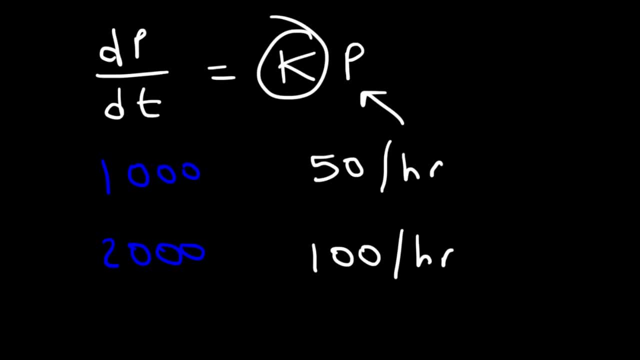 The rate at which the population grows is proportional to the population size. So if you increase the population size, dp by dt will increase proportionally. If you double the population size, the rate will double. If you triple it, the rate will triple. 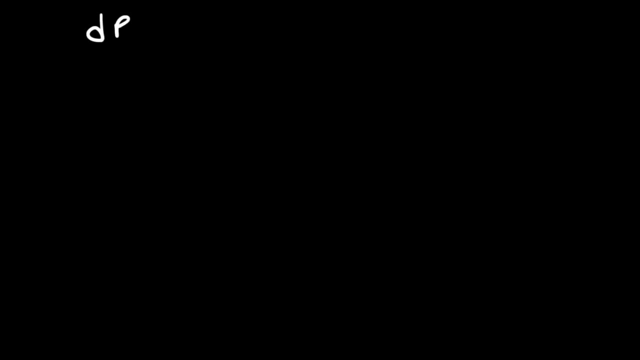 Now from that equation, how can we derive a general formula to calculate the population at any time? t? In order to do this, let's multiply both sides by dt, so that these two will cancel, and so we have: dp is equal to kp times dt. 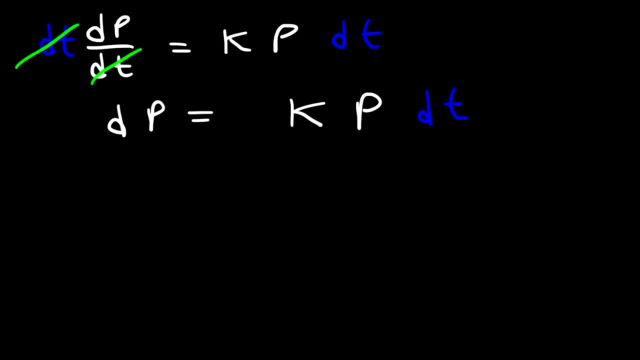 Now we need to separate the variables. k is a constant, As we said. it's the relative growth rate. We need to separate p from dt, So let's divide both sides by p. So now we have this expression: 1 over p dp is equal to k- dt. 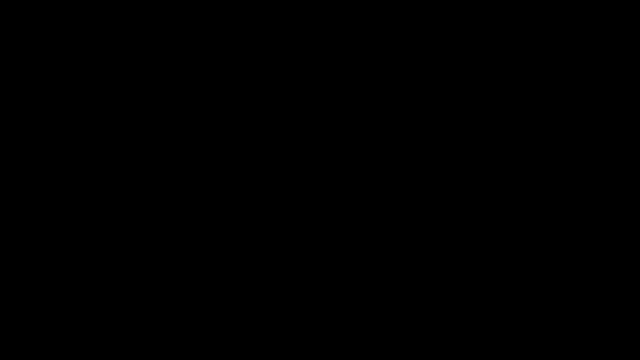 In this video, we're going to talk about exponential growth and decay problems as it relates to population growth, so to speak. Now, the first equation you need to be familiar with is this equation: dp divided by dt is equal to k times p. 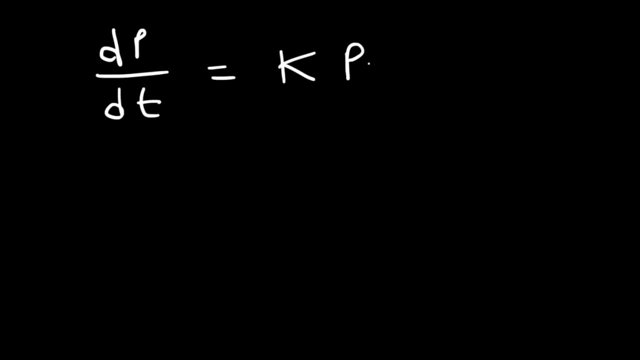 So this equation tells us that the population grows at a rate that is proportional to the size of the population. The population growth rate is dp by dt. That's how fast the population is growing at a given time. k is the relative growth rate and p is the size of the population at some time t. 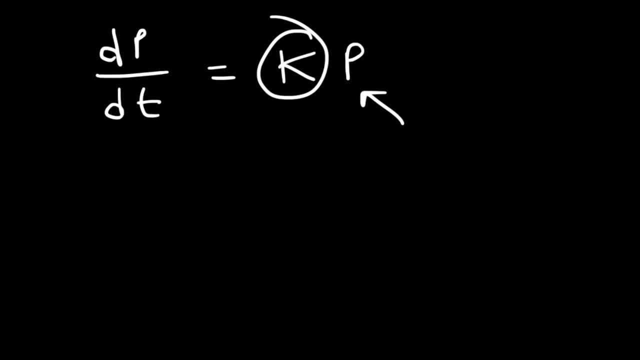 Now to understand this conceptually. let's say if we have a sample of a thousand bacteria, Okay, And let's say that in this sample the bacteria grows 50 cells per hour. What's going to happen if we double the population? 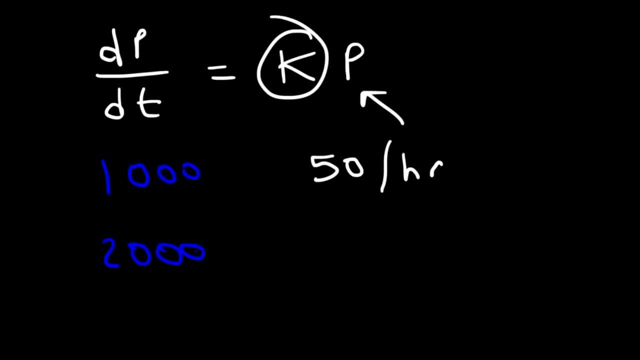 Let's say, if we have a sample of 2,000 bacteria counts, Well, since we have twice the amount of bacteria, we should expect it to grow at twice the rate, That is, at 100 cells per hour. So thus we could see that. 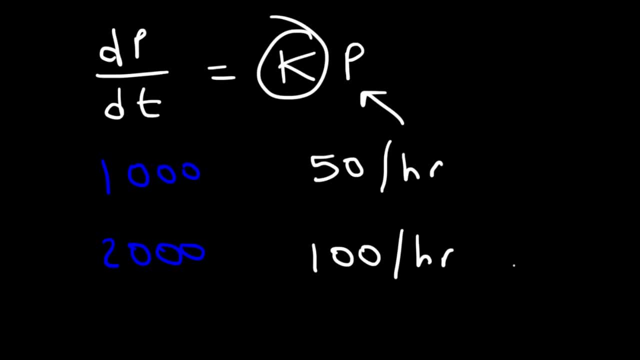 The rate at which the population grows is proportional to the population size. So if you increase the population size, dp by dt will increase proportionally. If you double the population size, the rate will double. If you triple it, the rate will triple. 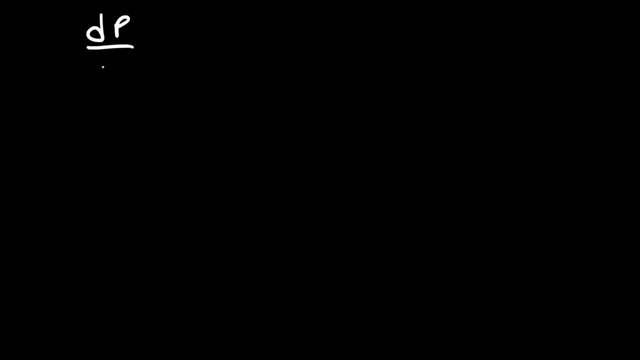 Now from that equation, how can we derive a general formula to calculate the population at any time? t? In order to do this, let's multiply both sides by dt, so that these two will cancel, And so we have: dp is equal to kp times dt. 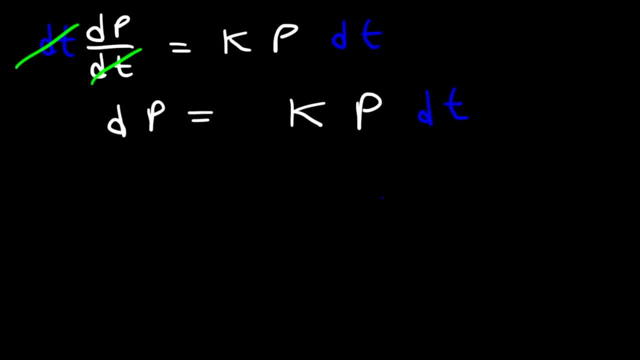 Now we need to separate the variables. k is a constant, As we said. it's the relative growth rate. We need to separate p from dt, So let's divide both sides by p. So now we have this expression: 1 over p dp is equal to k- dt. 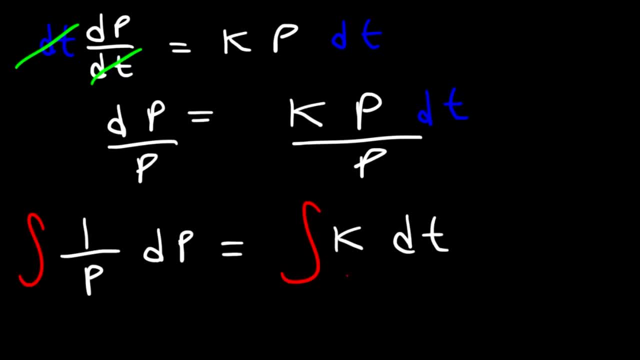 So at this point let's integrate both sides. The antiderivative of 1 over p is simply the natural log of p. k is a constant. The antiderivative of dt is t, So this is going to be k times t plus the general constant c. 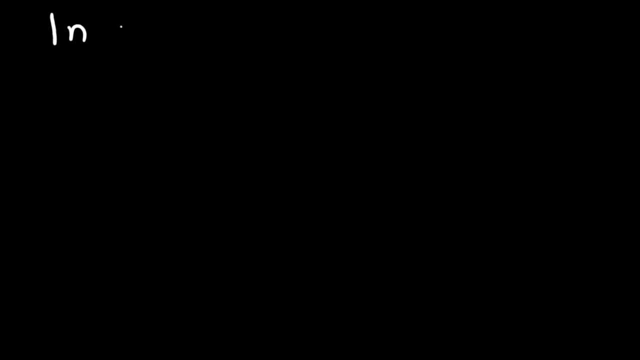 So this is going to be k times t plus the general constant c. So what should we do at this point, Now that we have this equation? How can we get p by itself? At this point, you want to put the equation on top of e, that is, on the exponent of e. 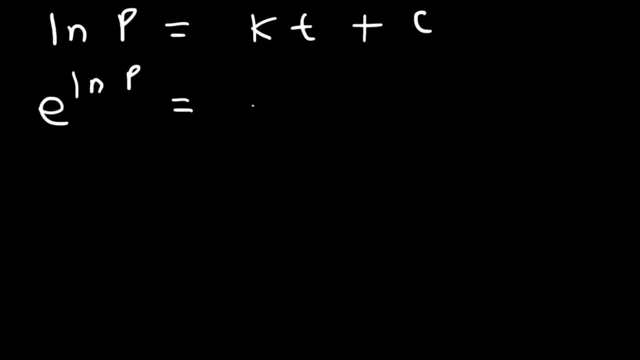 If ln p is equal to kt plus c, then e raised to the ln p is equal to e raised to the kt plus c. Now the base of a natural log is base e. Now the base of a natural log is base e. So these two will cancel. 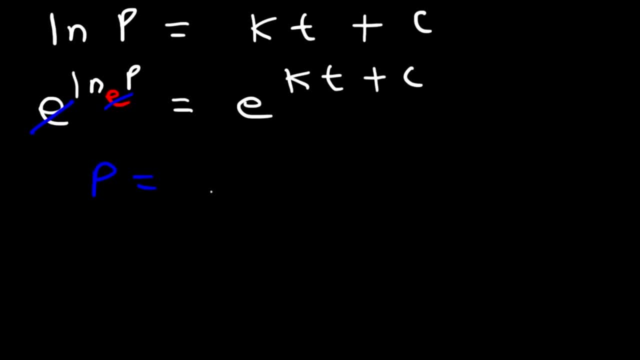 And so p is equal to e raised to the kt plus c. Now just to review some things in algebra, You know that x squared times x cubed is equal to x to the fifth. What you need to do is you need to add the two exponents. 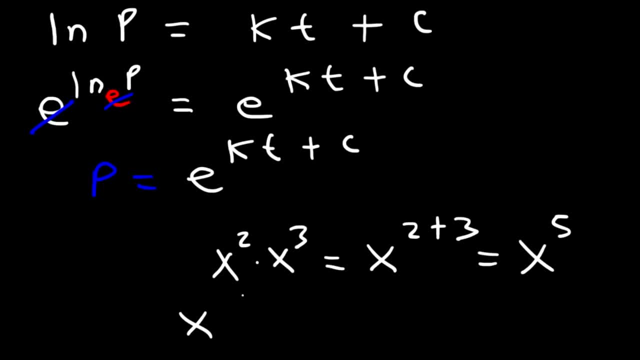 So what if we work backwards? We could say that x raised to the 4 plus 7.. We could say that x raised to the 4 plus 7. Is equal to x to the 4th times x to the 7th. 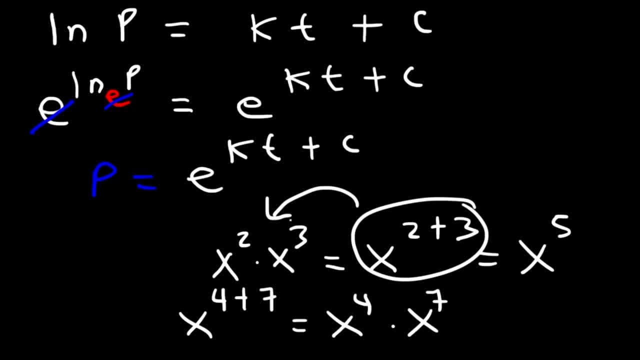 Basically, we're starting here and going back to this form. Notice that kt is added to c. So therefore, what we could do is we could say that e to the kt plus c is equal to e raised to the kt times e to the c. 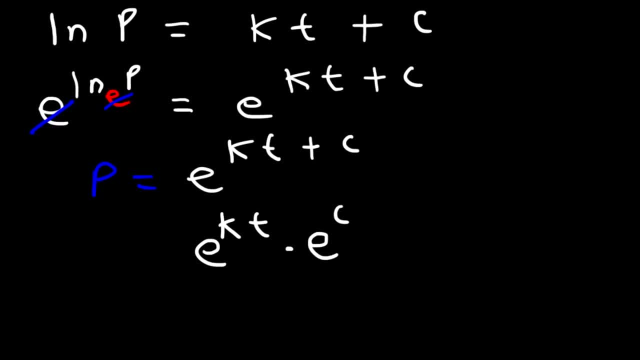 Now, e to the c is a constant, So we can simply replace it with c. So the population is equal to c, e to the kt. So the population is equal to c, e to the kt. Now, starting with this equation, We're going to calculate p of 0.. 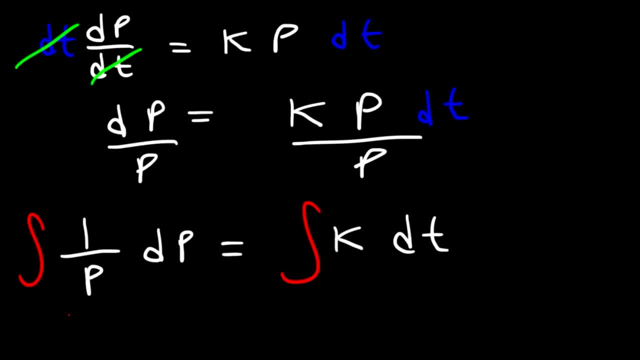 So at this point let's integrate both sides. The antiderivative of 1 over p is simply the natural log of p. k is a constant. The antiderivative of dt is t, So this is going to be k times t plus the general constant c. 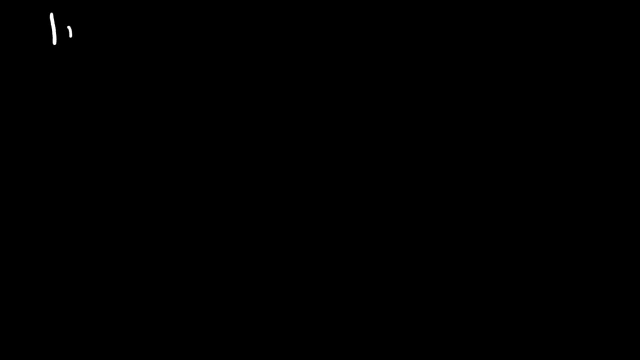 So what should we do at this point, now that we have this equation, How can we get p by itself? At this point? you want to put the equation on top of e, that is, on the exponent of e. If lnp is equal to kt plus e, then e raised to the lnp is equal to e raised to the kt. 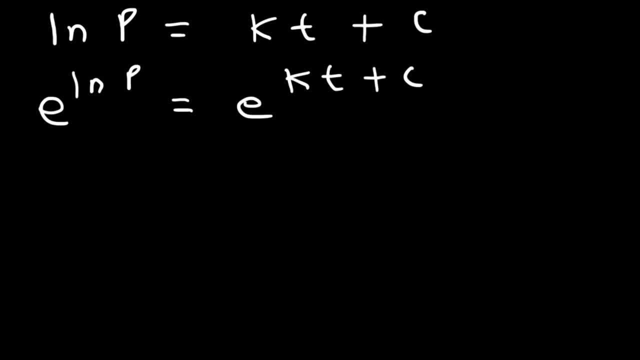 plus c. Now the base of a natural log is base e, So these two will cancel. And so p is equal to e raised to the kt plus c. Now just to review some things. in algebra you know that x squared times x cubed is equal. 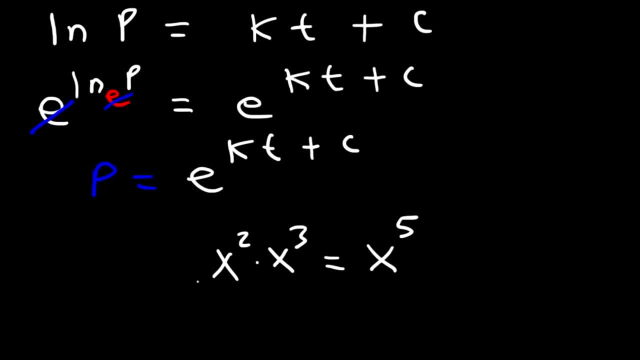 to x to the fifth. What you need to do is you need to add the two exponents. So what if we work backwards? Let's do that. We could say that x raised to the fourth plus seven is equal to x to the fourth times. 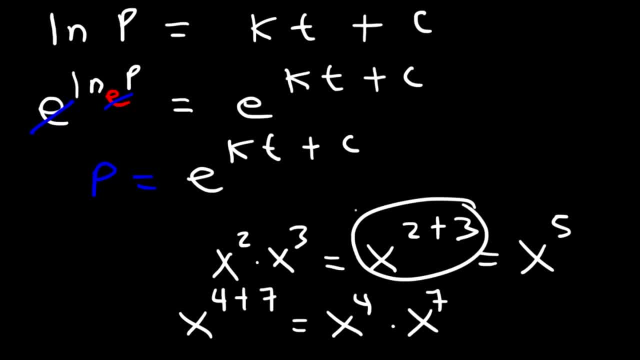 x to the seventh. Basically, we're starting here and going back to this form. Notice that kt is added to c. Therefore, what we could do is we could say that e to the kt plus c is equal to e raised to the kt times e to the c. Now e to the c is a constant, so we could simply replace it with c, So the 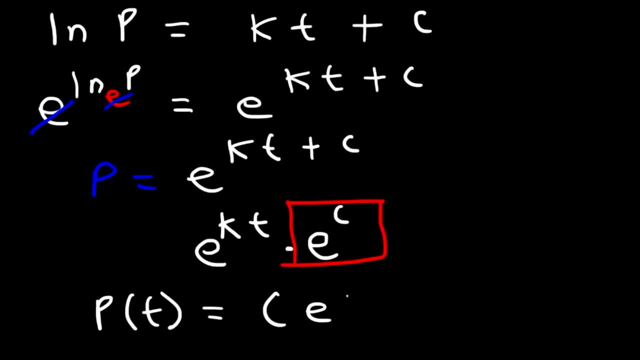 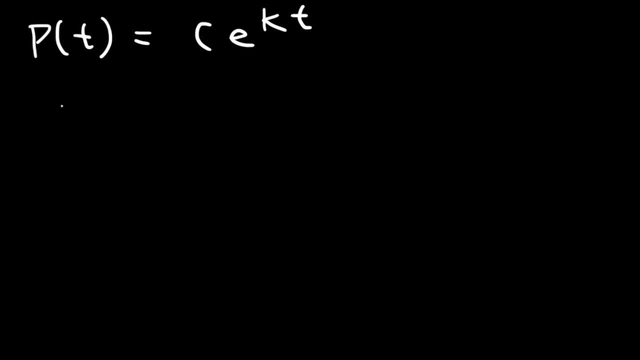 population is equal to ce to the kt. Now, starting with this equation, we're going to calculate p of zero. So let's replace t with zero. This is going to be ce k times zero. k times zero is simply zero. So this is going to be ce to the zero. Now, anything raised to the zero, 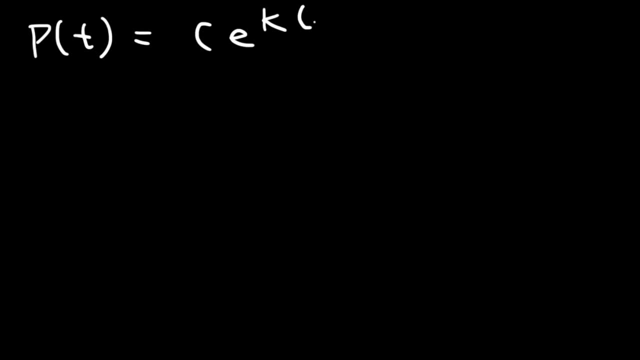 We're going to calculate p of 0.. 0.. So let's replace T with 0. This is going to be c? e k times 0.. k times 0 is simply 0. So this is going to be c? e to the 0.. Now anything raised to the 0. 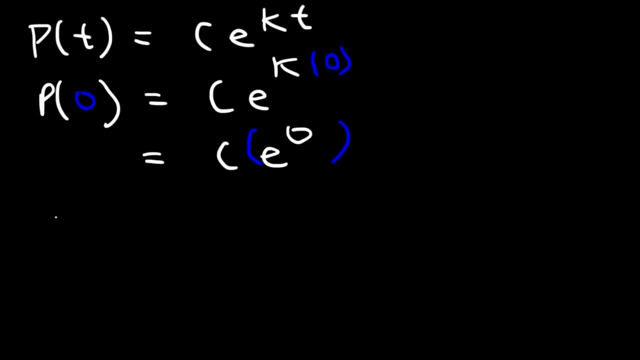 power is equal to 1.. So therefore p of 0 is c times 1.. So c is the initial value. It's the population at t equals 0. So we could say c is basically p initial. Thus we can replace c with p initial. So the general equation is the population at. 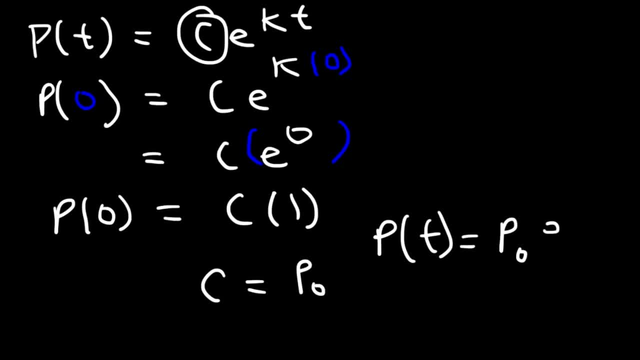 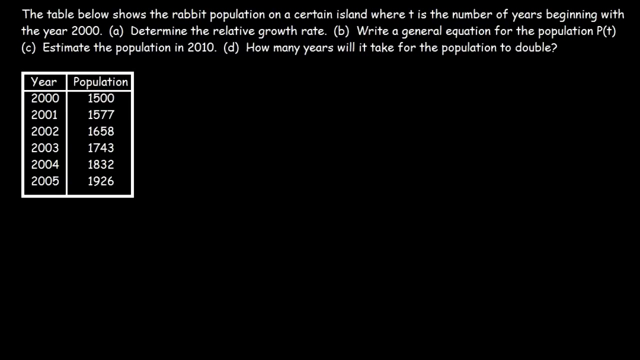 any time, t is equal to the initial population, p, 0, e times the relative growth rate, which is k multiplied by t. So now you know how to derive this formula from this expression. Let's work on this problem. The table below shows the rabbit population on a. 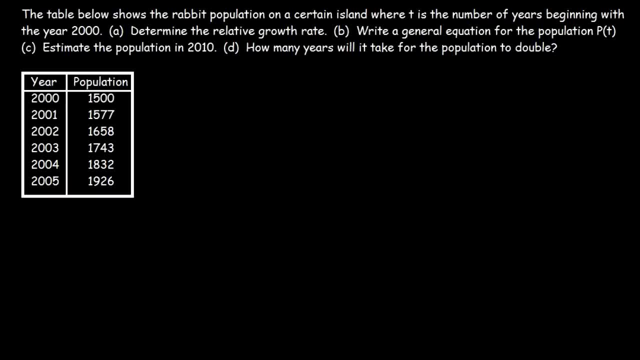 certain island where t is the number of years beginning with the year 2000.. Determine the relative growth rate. So we need to use the equation: p of t is equal to p of 0, e raised to the kt. Our goal is to solve for k, But 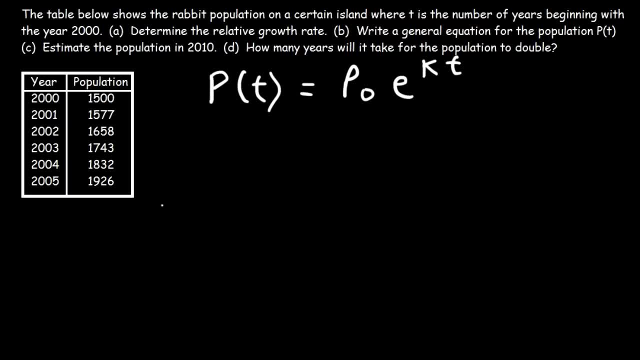 first we gotta find p 0. So what exactly is p 0?? Well, p of 0 is equal to 1500.. When t is 0, that is the year 2000,. the population is 1500. So which is the result we pick? When t is equal to 15000, the population is 1500.. Just enter the line. 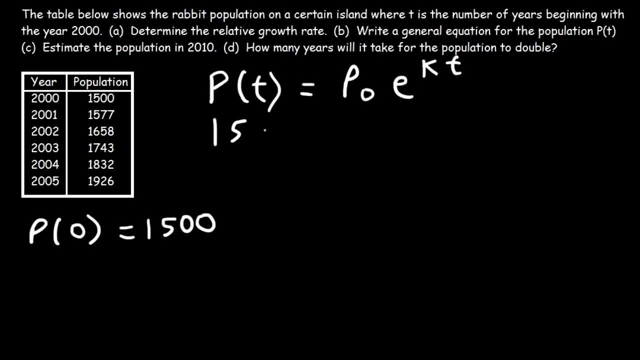 Can we play along? Yes, Can we play along? Let's do it again. Yes, Let's play along. So if we replace P of T with 1500 and T with 0, we're going to get 1500 is equal to P0. 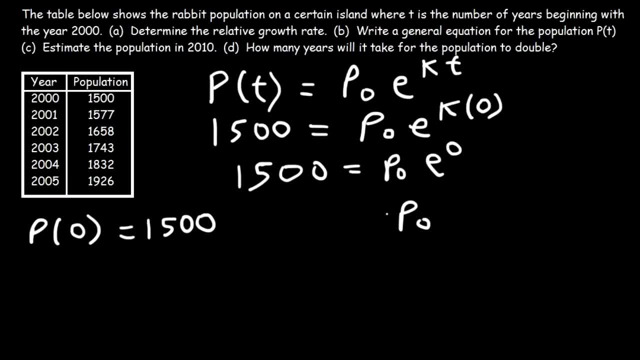 e to the 0.. e to the 0 is 1, so P0 is 1500.. So P of 0 is the same as P sub 0.. That's the initial population. So how can we use this to calculate K? 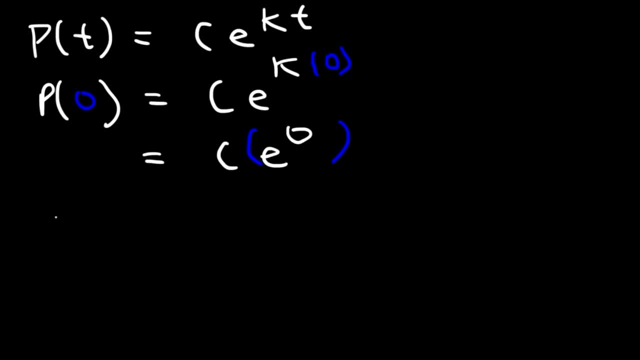 power is equal to one. So therefore p of zero is c times one. So c is the initial value. It's the population at t equals zero. So we could say c is basically p initial. Thus we can replace c with p initial. So the general equation is the population. 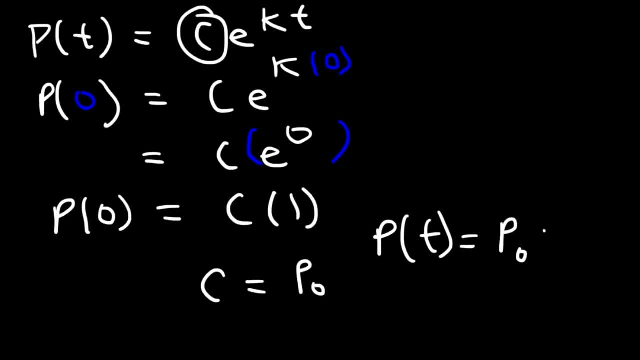 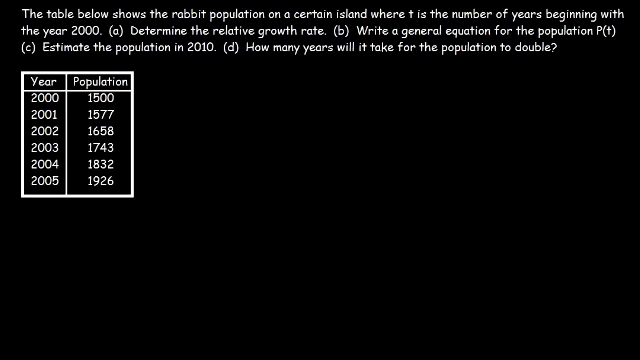 at any time, t is equal to the initial population, p zero, e times the relative growth rate, which is k multiplied by t. So now you know how to derive this formula from this expression. Let's work on this problem. The table below shows the rabbit population on a certain island. 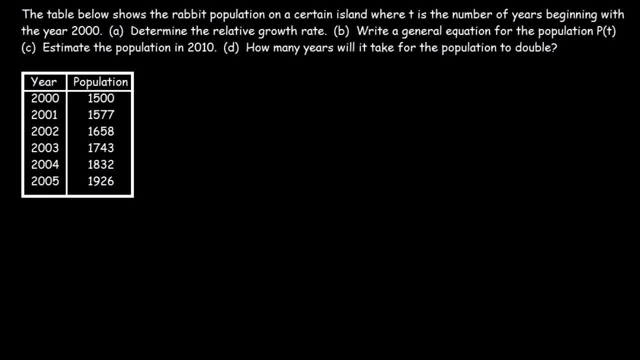 where t is the number of years beginning with the year 2000.. Determine the relative growth rate. So we need to use the equation: p of t is equal to p of zero, e raised to the kt. Our goal is to solve for k, But first we have to find p zero. So what exactly is p zero? 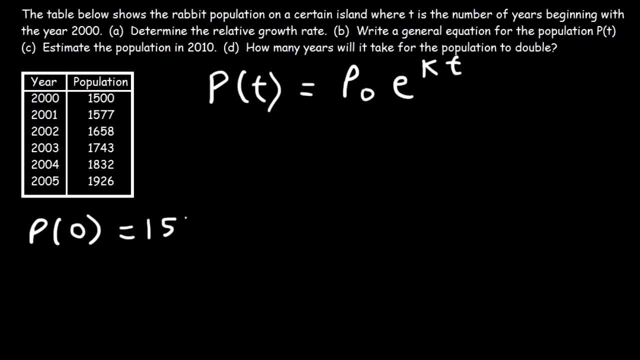 Well, p of zero is equal to fifteen hundred. When t is zero, that is the year 2000,. the population is fifteen hundred. So if we replace p of t with fifteen hundred and t with zero, we are going to get fifteen hundred is equal to p zero, e to the zero. e to the zero is. 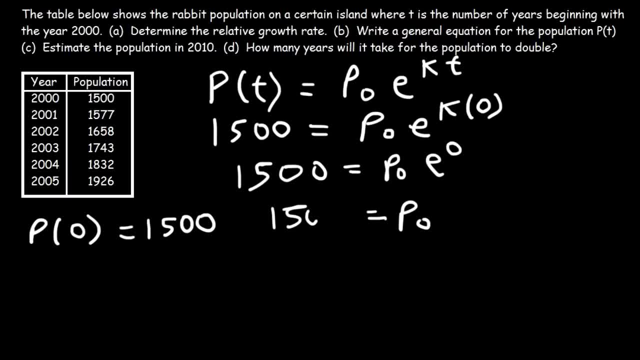 one. so p zero is fifteen hundred. So p of zero is the same as p sub zero. That is the initial population. So how can we use this to calculate k? So now that we have the value of p of zero, we can say that p of t is fifteen hundred. 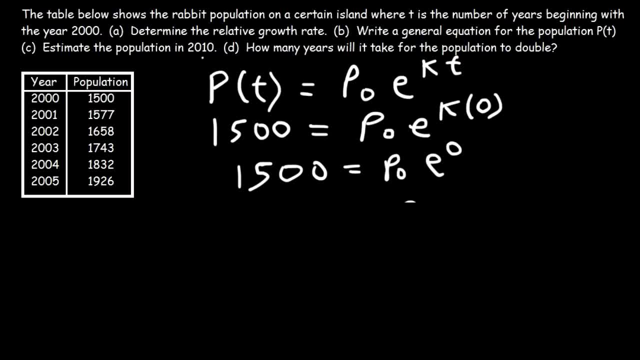 So now that we have the value of P of 0, we can say that P of T is 1500, that's P0, e KT. So now let's use another point to calculate K. We can use any point in the data table, but let's use the first one. 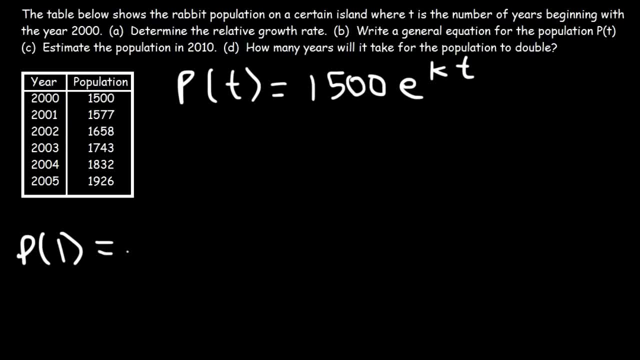 In the year 2001,. T is equal to 1.. So the population at T equal 1 is 1577.. So let's replace P of T with 1577, and let's replace T with 1.. In order to solve for K, let's divide both sides by 1500. 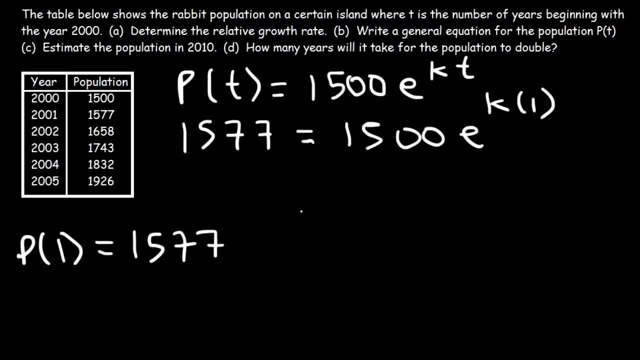 1577 divided by 1500.. 1500 is equal to 1.0513.. And that's equal to e raised to the K power. So now, at this point, we need to take the natural log of both sides, The natural log of e to the K. what do you think that's equal to? 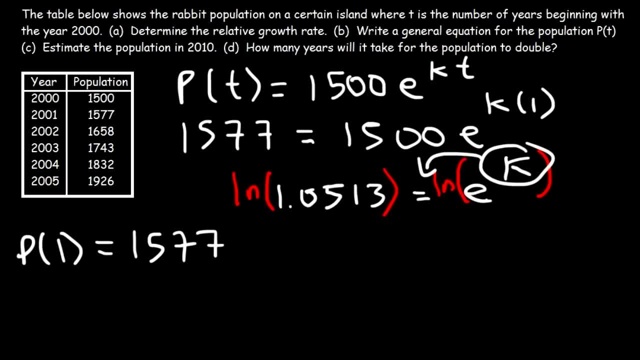 A property of logs allows us to move the constant or the exponent to the front. So this is equal to E. So this is equal to K times the natural log of E. The natural log of E is equal to 1.. So K is simply equal to ln 1.0513.. 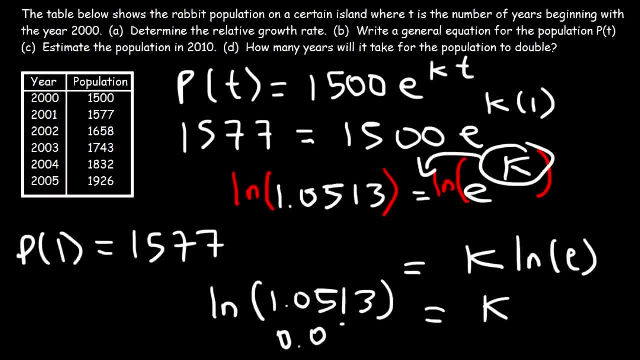 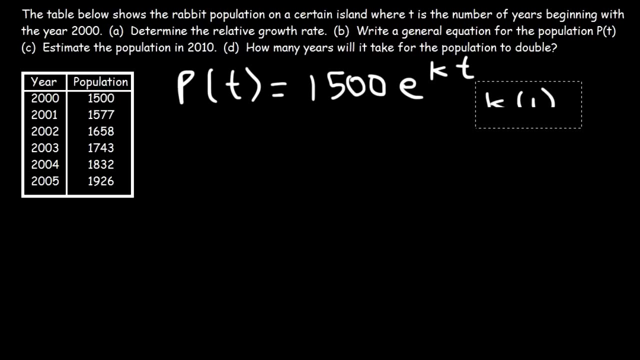 Which is about 0.05.. So that's the value of K. So now we can write a general formula. So to write the general formula, it's going to be 1500 E, and then all we need to do is 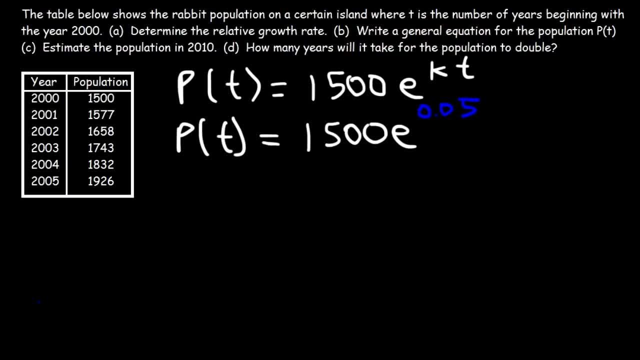 replace K with 0.05 times T. So that's the answer to part B. That's the general equation that will give you the population P of T at any time T. The answer to part A: the relative growth rate is the value of K, which is 0.05.. 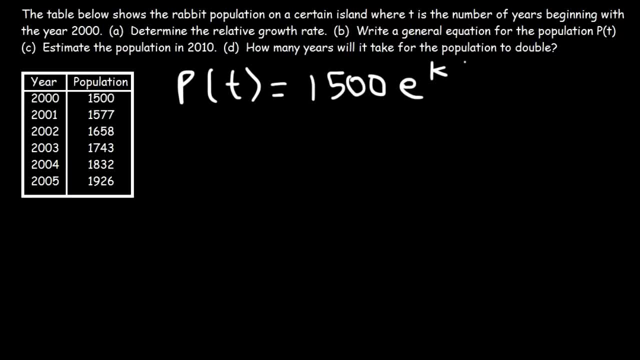 that is, p, zero, e, kt. So now let's use another point to calculate k. We can use any point in the data table, But let's use the first one In the year 2001,. t is equal to one, So the population at t equal one is fifteen, seventy-seven. So let's replace p of t with. 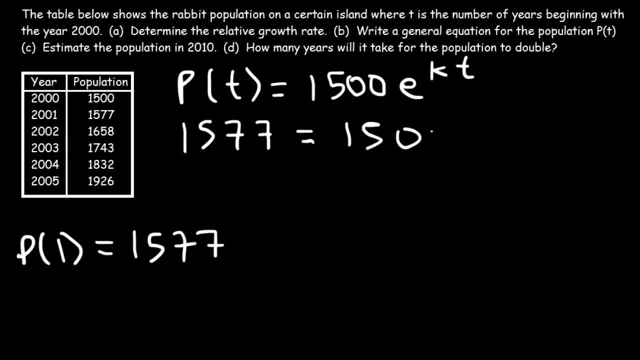 fifteen seventy-seven, and let's replace t with one In order to solve for k. let's divide both sides by fifteen hundred. Fifteen seventy-seven divided by fifteen hundred is equal to one point zero, five, one, three, And that's it. 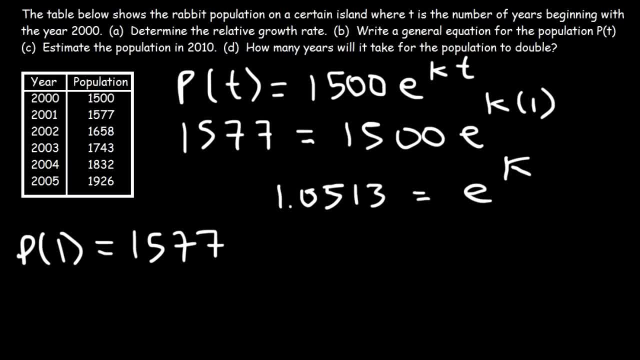 That's equal to e raised to the k power. So now, at this point, we need to take the natural log of both sides, The natural log of e to the k. what do you think that's equal to? A property of logs allows us to move the constant or the x-point into the front. So this is: 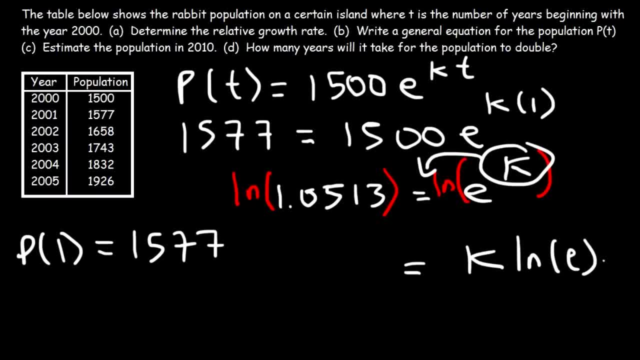 equal to k times the natural log of e. The natural log of e is equal to one. So k is simply equal to ln. one point zero five. one three, Which is about point zero five. So that's the value of k. So now we can write a general formula. 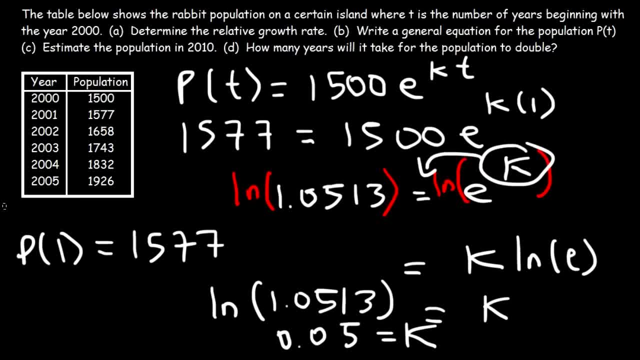 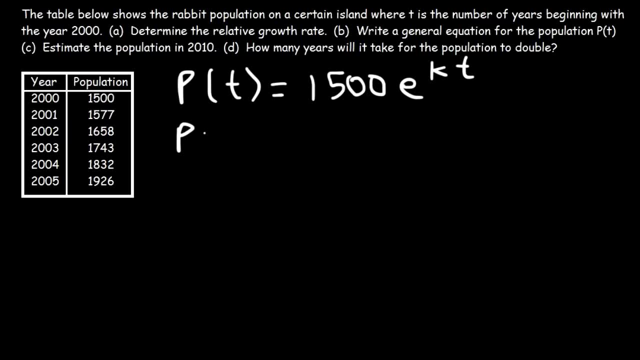 So now we can write a general formula. So to write the general formula, it's going to be fifteen hundred e, and then all we need to do is replace k with point zero, five times t. So that's the answer to part b, That's the. 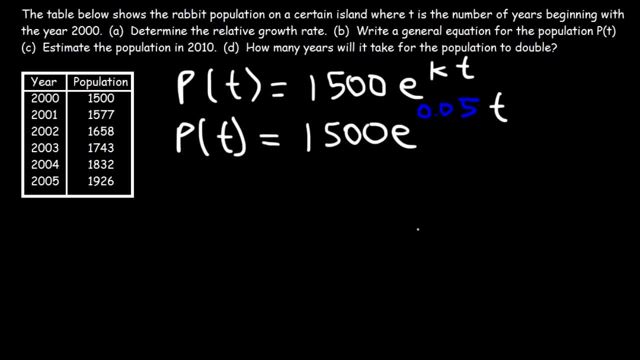 general equation that will give you the population p of t at any time. t. The answer to part b is part a. the relative growth rate is the value of k, which is point zero five. So basically, the population increases by five percent every year, compounding continuously This formula. 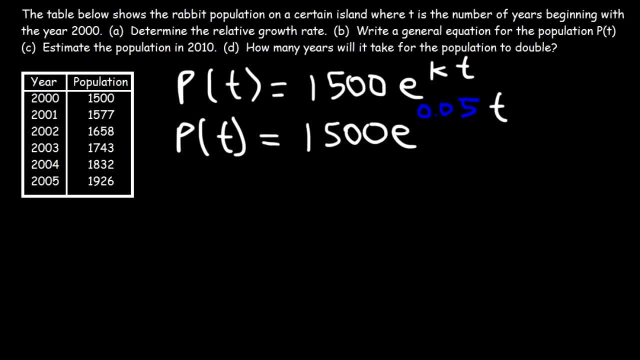 So, basically, the population increases by 5% every year, compounding continuously. This formula is the general formula of the compound interest type problem. Now how can we estimate the population in 2010?? To do that, simply replace T with 10.. 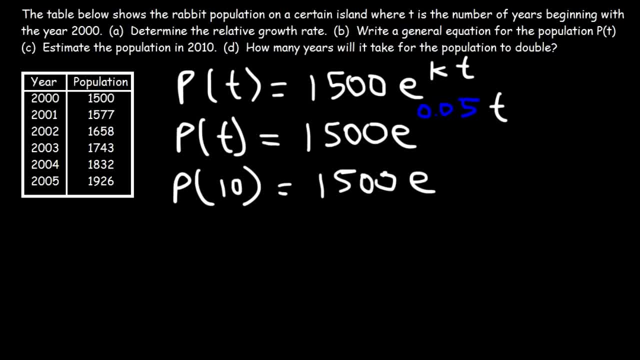 So this is going to be 1500 E raised to the 0.05 times 10.. And just type it in your calculator exactly the way you see it: 0.05 times 10 is 0.5.. So it's 1500 times E raised to the 0.5.. 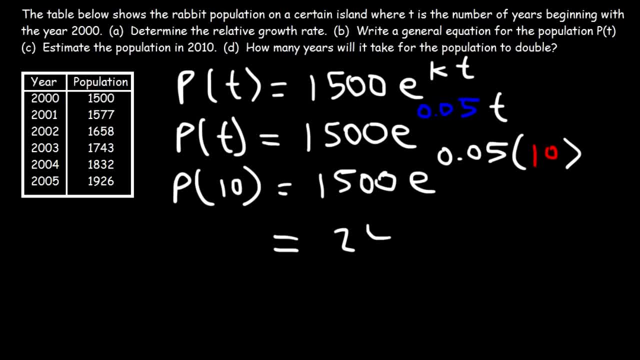 And so the population is going to be about 2,473 rabbits in the year 2010.. Now, how many years will it take the population to double? And that's starting from the year 2000.. What we're going to do is we're going to find out how long it takes for the population to double from. 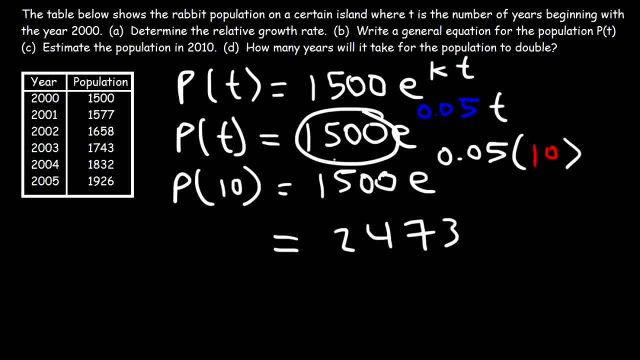 1500 to 3,000, because 1500 times 2 is 3,000.. So let's replace P of T with 3,000.. And we just got to solve for the variable T, So let's get rid of a few things. 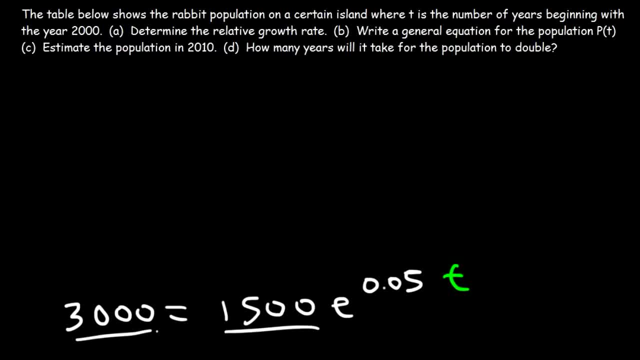 So our first step is to divide both sides by 1,500.. 3,000 divided by 1,500 is simply 2.. So 2 is equal to e raised to the .05 times t. Next we need to take the natural log of both sides. This will allow us to take this: 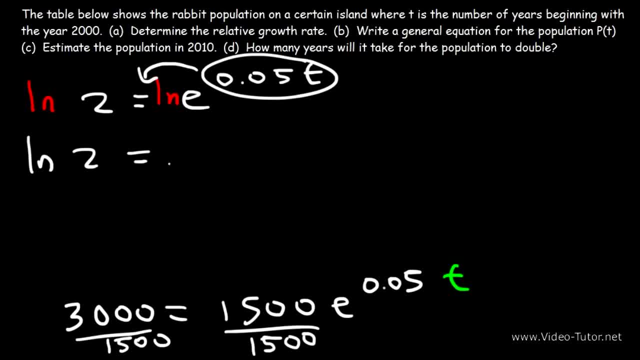 exponent and move to the front. So the natural log of 2 is equal to .05 times t multiplied by the natural log of e, And the natural log of e is 1.. So ln 2 is equal to .05 times t. So the time it takes for it to double is simply ln 2 divided by the rate constant k. 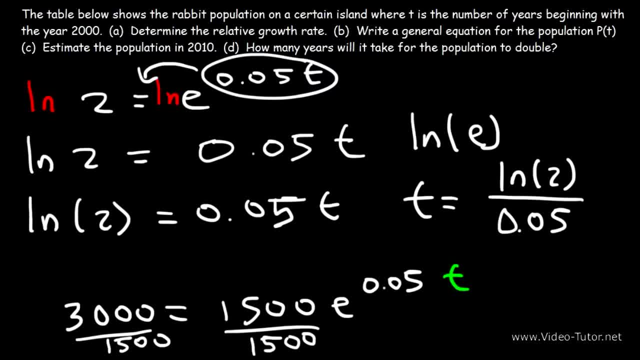 the relative growth rate. So if we divide these two numbers, ln 2 is like .6931 divided by .05.. So it's going to take .0931 divided by .0931.. So it's going to take .0931 divided by .0931.. 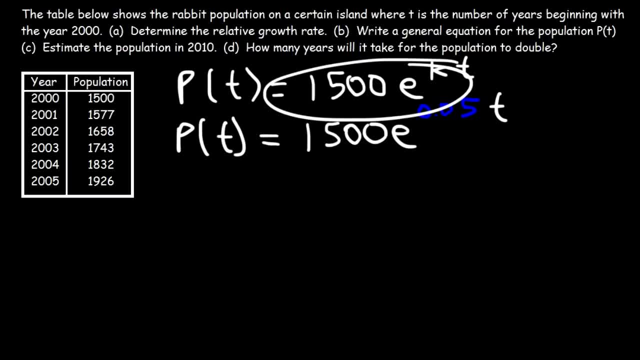 is the general formula of the compound interest type problems. Now how can we estimate the population in twenty ten? To do that, simply replace t with one point zero, five times t. So that's the general formula. Let's start with t, with ten. 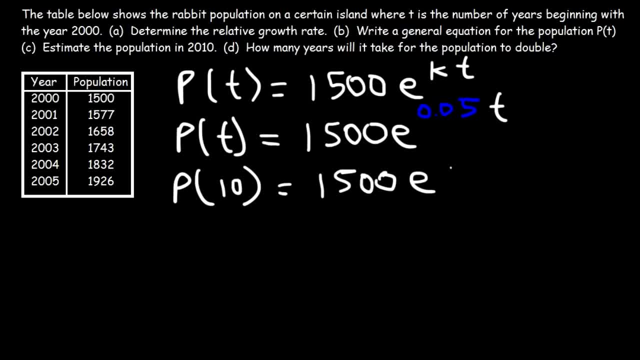 So he's going to be fifteen hundred e raised to the point zero, five times ten. And just type it in your calculator exactly the way you see it. Point zero five times ten is point five. So it's fifteen hundred times e raised to the. 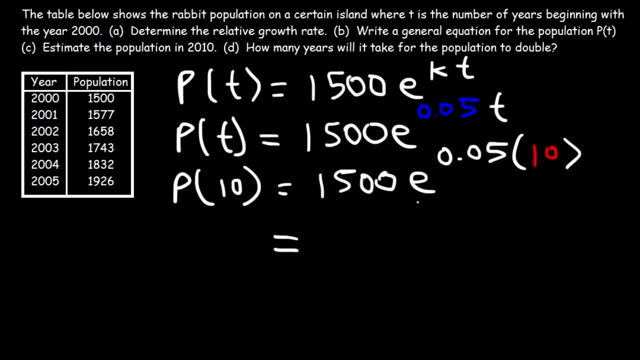 point five. And so the population is going to be about two thousand four hundred and seventy three in the year 2010. now, how many years will it take the population to double? and that's starting from the year 2000. what we're gonna do is: we're gonna find out. 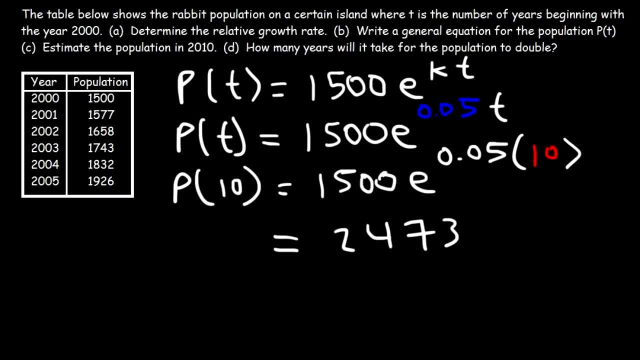 how long it takes for the population to double from 1500 to 3000, because 1500 times 2 is 3000. so let's replace PFT with 3000. and we just got to solve for the variable T, so let's get rid of a few things. 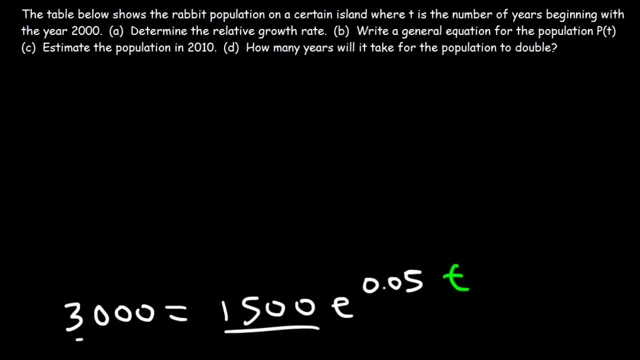 so our first step is to divide both sides by 1500. 3000 divided by 15 hundred is simply 2, so 2 is equal to e raised to the point 0, 5 times T. Next, we need to take the natural log of both sides. this will allow us to take this: 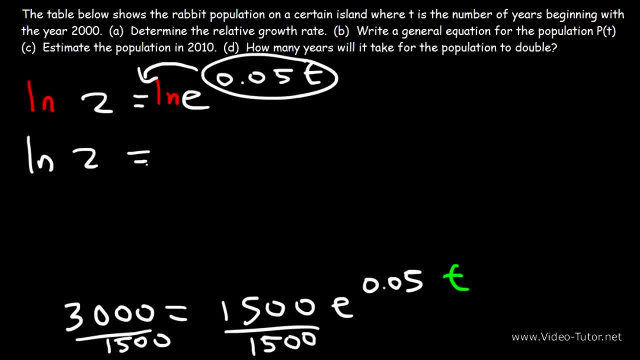 exponent move to the front. so the natural log of 2 is equal to 0.5 times T multiplied by the natural log of E. and the natural log of E is 1, so ln 2- LN2 is equal to 0.05 times T. 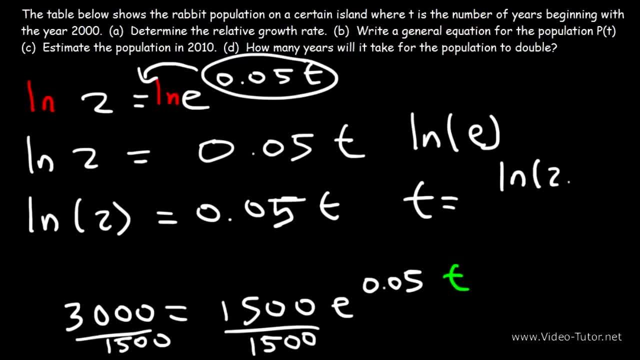 So the time it takes for it to double is simply LN2 divided by the rate constant K, the relative growth rate. So if we divide these two numbers, LN2 is like 0.6931 divided by 0.05.. So it's going to take 13.86 years in order for the population to double.